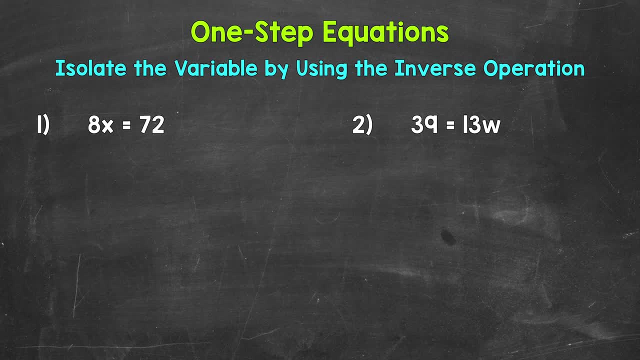 Anytime you see a number next to a variable, that is multiplication. So something to keep in mind. Now we need to isolate that variable of x. We need to figure out what x equals. Since x is being multiplied by 8, we need to undo that multiplication by using the inverse operation. 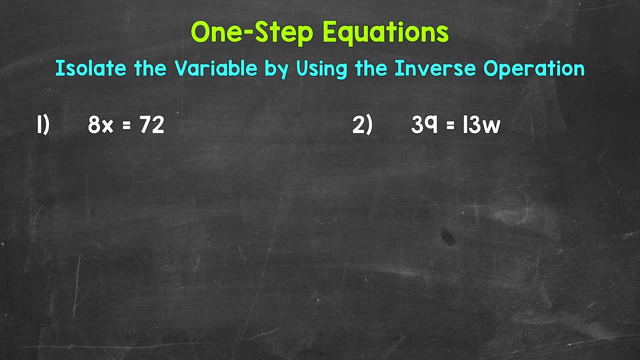 So the opposite operation, The opposite of multiplication, is division. So let's divide the left side of the equation by 8.. Now, whatever we do to one side of the equation, we must do to the other in order to keep it balanced and equal. 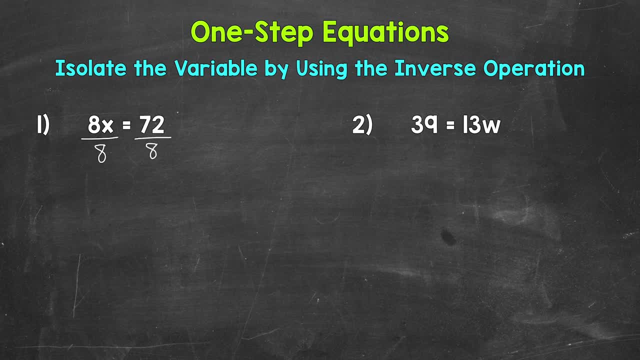 So let's divide the right side by 8 as well. Now, as far as the left side of the equation, we are multiplying by 8 and dividing by 8. So these are equal. These 8s cancel each other out. 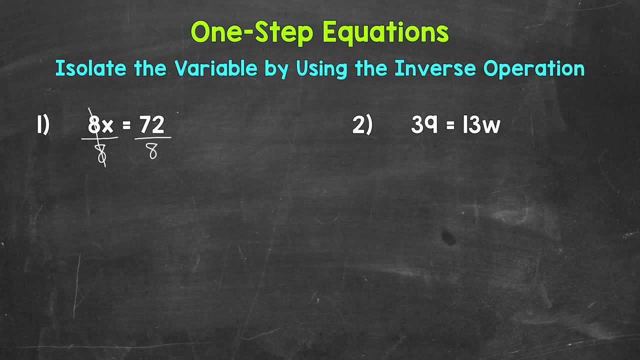 We have 8 divided by 8. That gives us 1.. So we have 1x, which is just x. Our variable of x is isolated, It's by itself. So we have x, equals 72, divided by 8, equals 9.. 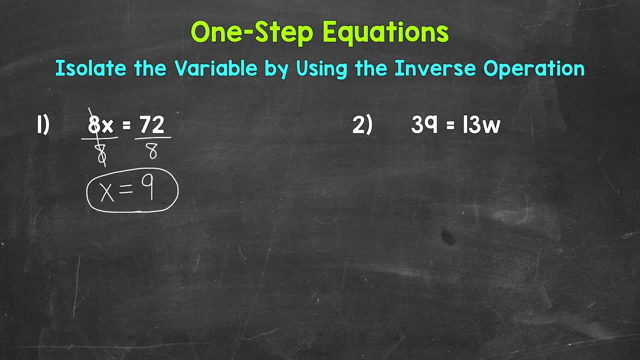 x equals 9.. That's our solution. Now we can always check a solution by plugging it in, Plugging it into the original equation. So let's plug 9 in for x and see if this works. We have: 8 times 9 equals 72.. 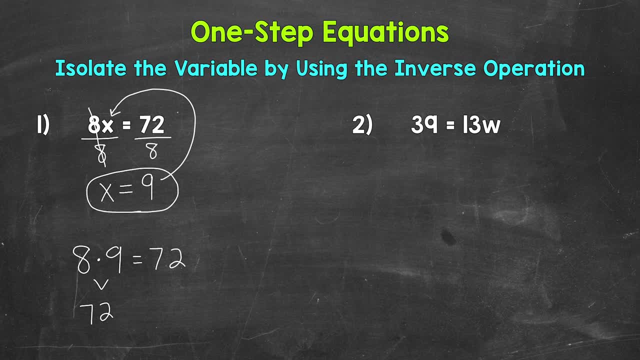 8 times 9 does equal 72. So we have the correct solution: x equals 9.. Now one thing I do want to mention about plugging that 9 back into the original equation: make sure to use something to represent the original equation. 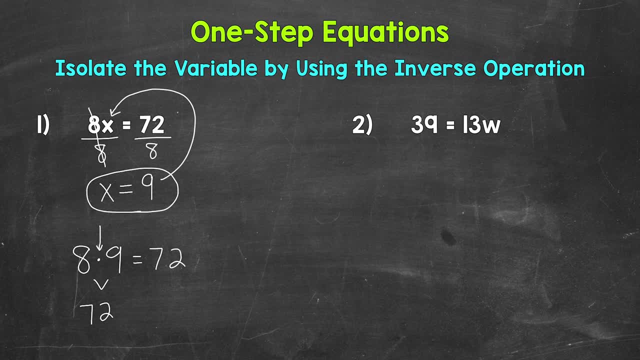 So let's plug 9 in for x. If I want to represent multiplication, I used a dot Putting the 9 right next to the 8, that would look like 89. Two numbers together does not represent multiplication, But when we have a number next to a variable, that does represent multiplication.